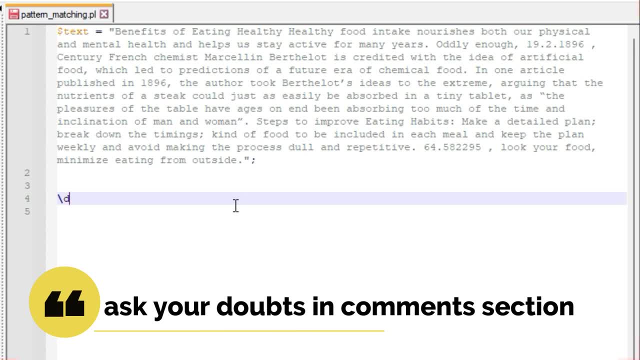 represent, but we do not know how many decimals it will be. So one or more decimals means we have to add plus after that. This particular pattern means there can be one or more integers in the paragraph Now, after that we have a dot. So if, after the date, if you see there is a dot here, So to represent, 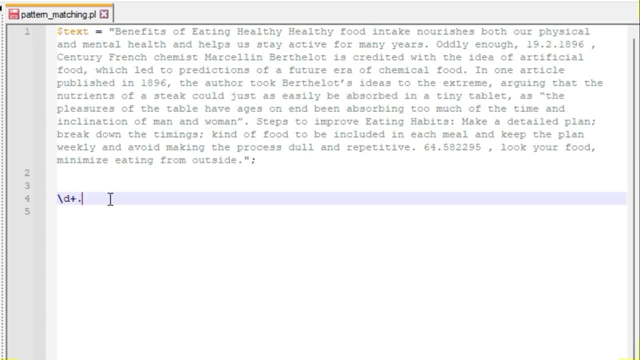 the dot. we have to put a dot like this, So after that we have a dot like this, So after that we have a dot like this, But tool will not understand. we have to add backslash before this. That will escape and then only Perl compiler will be able to understand that there is a dot and we have to. 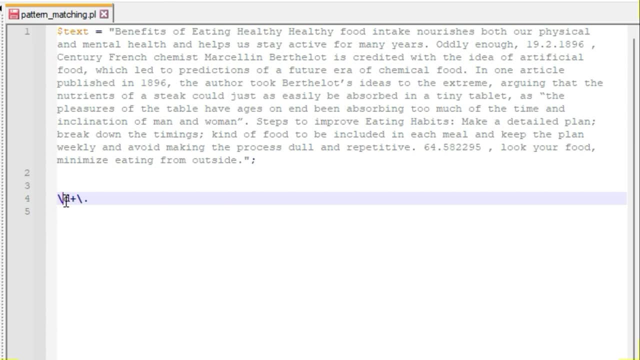 match this pattern. So this pattern represents that there is one or more integers, and after that there is a dot, and after that again there will be one or more integers. So this particular pattern will be repeated again, and after that there is a dot, and after that again. we need 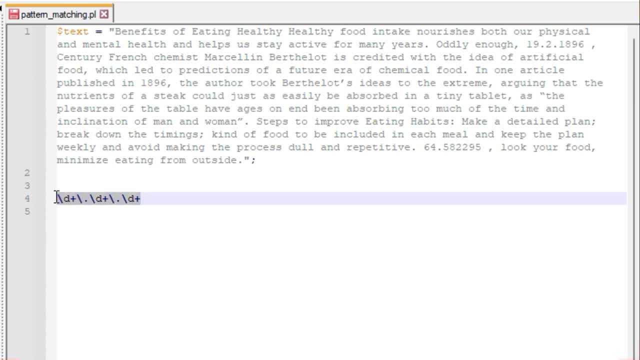 one or more integers like this. So this particular pattern means this is your matching pattern with the date, and to complete the pattern we have to put it in the parenthesis. So if we put it in parenthesis like this, this becomes the full pattern and after this we will put it in the 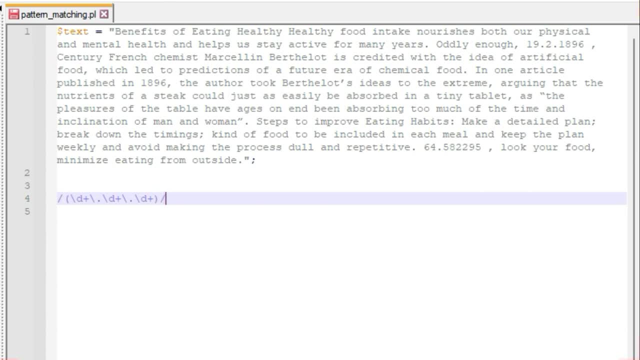 forward slashes like this. Specifying like this means this is now a full pattern which has to be searched In the text variable. So if you see here, variable is this, that is text variable. So we name the variable like this and after that, if we put it like this, So this, equal to and tilde, means that 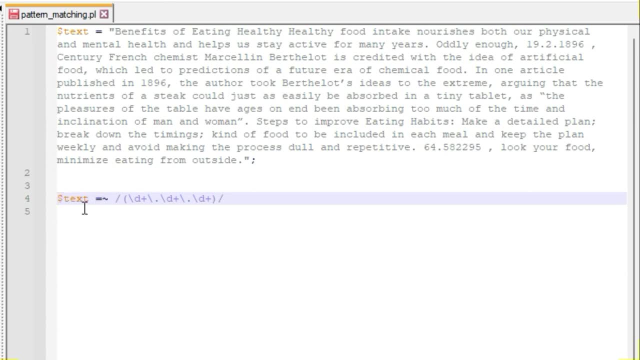 you are asking the tool or your compiler to search for this particular pattern in this string. So this will be a variable. and then we put it in the parenthesis again, Like this. Then it becomes a full regular expression. That is, you are asking the 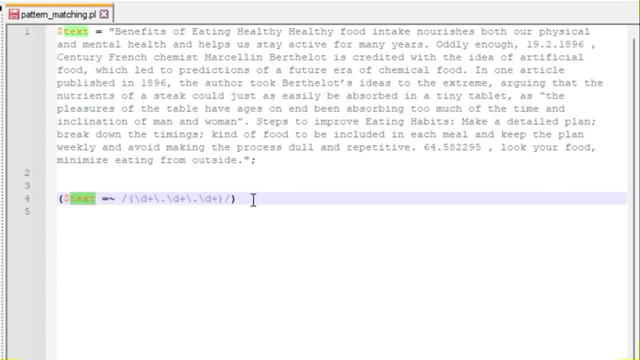 Perl compiler to search for this particular string in this pattern with this pattern. So this is now full and we have to assign it to something. So we are saying that this is our date and once this date is complete, now you can save it and we can try to run it Now if you simply go and run it, 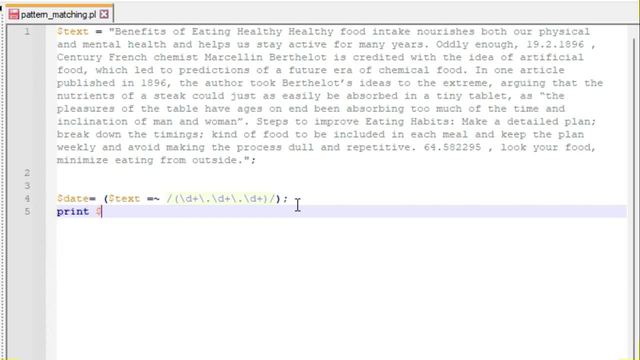 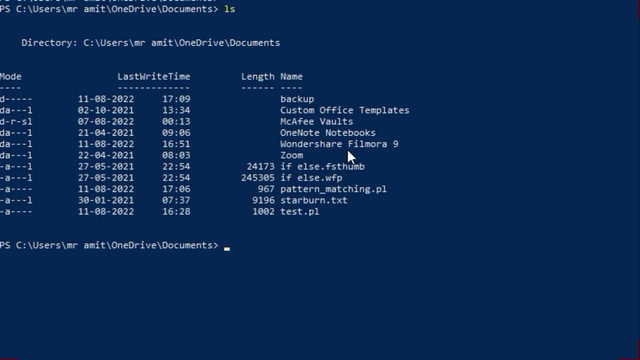 it will not run because there is no print command. So first we need to write print date here. Then only we will be able to run it and see the output. All right, this is the command line. So if we do ls, we can see that this is the file name. Now, if we do, 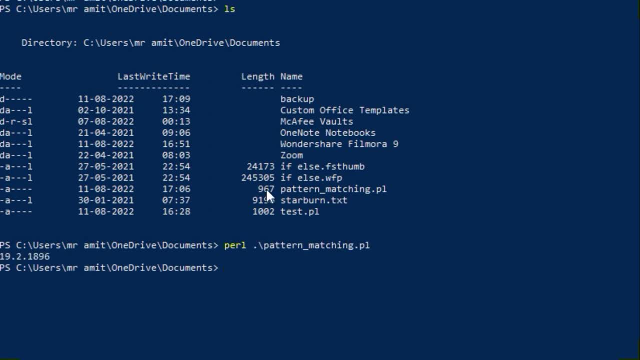 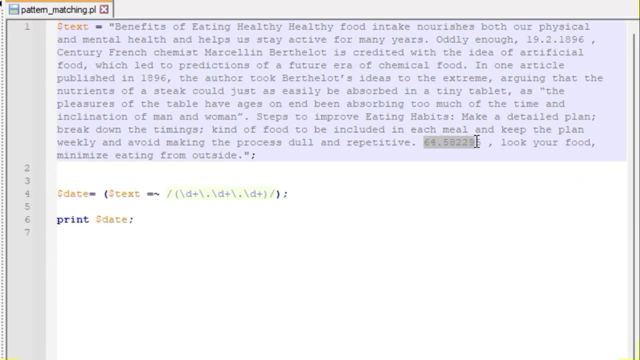 Perl and then pattern matching, So you can see that date is correctly getting extracted here. Now coming back to our next task. Next task is to extract the phone number, and we know that there is one decimal in between, two decimals, two digits before the decimal. 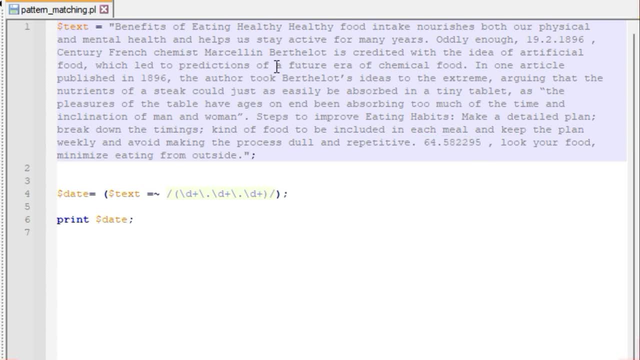 And six digits after the decimal. that is the pattern and we have to extract it. We don't know the position of this pattern, So what we can do is we know that one integer represents backslash d, So backslash d, and after that we know that one or more is represented by plus, But we need a. specific count, that is two digits before the decimal. So that can be specified like this in curly braces: That means that two or more digits can two digits. So exactly it will match, not two or more, not one. It will exactly match two digits only. And after that our pattern is dot and that we specify with the escape sequence like this: And after that we need again integers, but we need exactly six integers after that. So this becomes our pattern now And this pattern we will specify in the brackets like this: 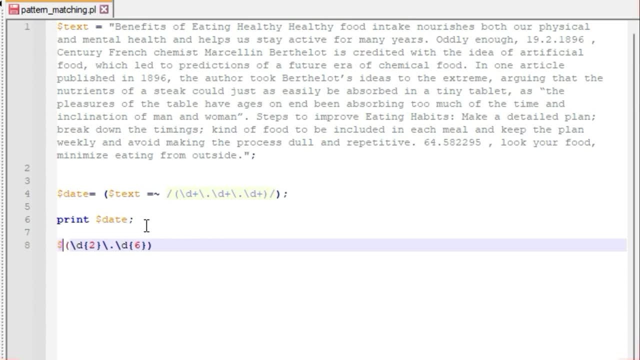 And after specifying like this, we have to search it In the text format. So again, variable is text. We specify it like this, and this is telling the compiler that we have to match this pattern and for matching it has to be specified in the forward. 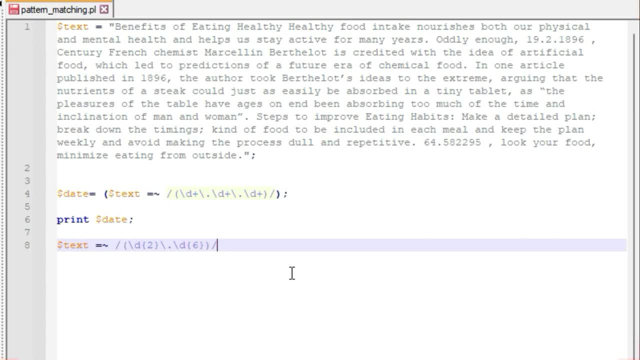 slashes like this. So this becomes your full regular expression, which should be in the parenthesis like this: And this is your final result and that has to be stored in some variable. So let's say phone is variable, in which we are storing it. After that we have to print it. So let's print like this phone and after that, variable phone. 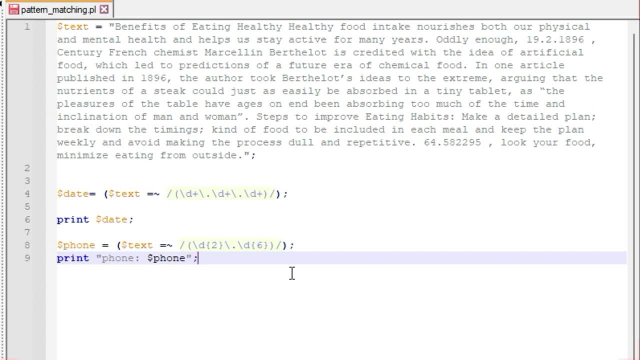 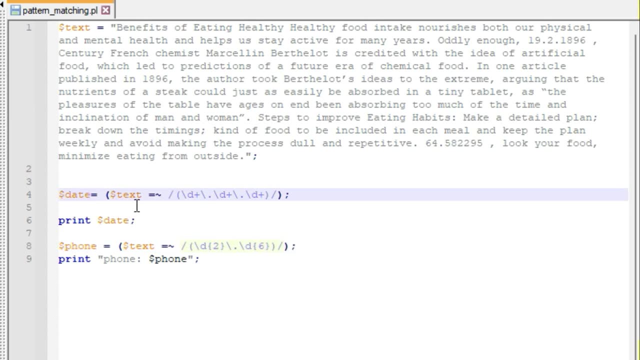 So this way you can search for phone number and we have to check whether it is correctly reflecting the output or not Before we go ahead and check first. please note that what happens sometimes is Perl compiler is not able to understand it correctly and assign the output.